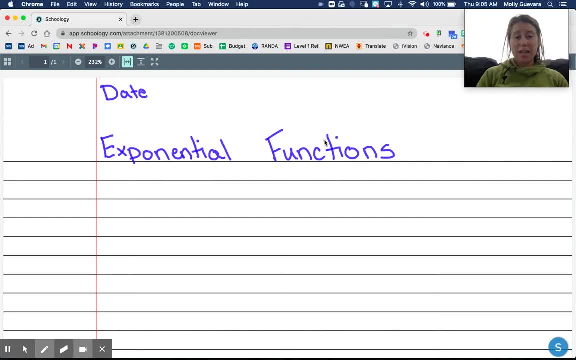 Hello everybody, welcome back. We're going to be taking notes on exponential functions today, So in your notebook make sure you date whatever today's date is and then write the title of the notes today, which is exponential functions. We're going to be going back and forth between some gluons and some. 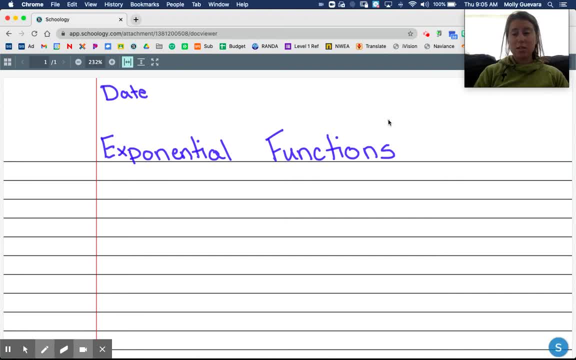 and writing in our notes today. So just be aware of that, Make sure you have your packet out or have whatever gluons you have access to out. Alright, so we're going to start with defining what is an exponential function. So an exponential function is in the form of. 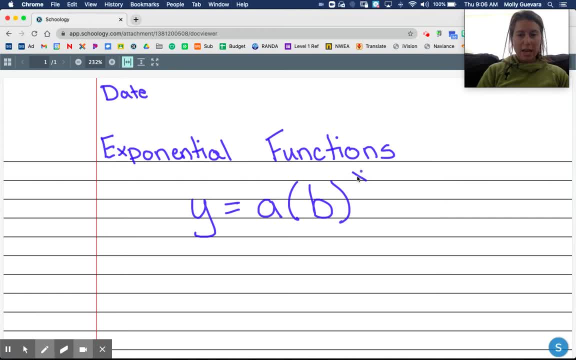 a times b to the x. Now, this is very important. The x has to be in the exponent. It cannot be down here in a. It cannot be down here in b. Okay, a. so the number in front of the base represents. 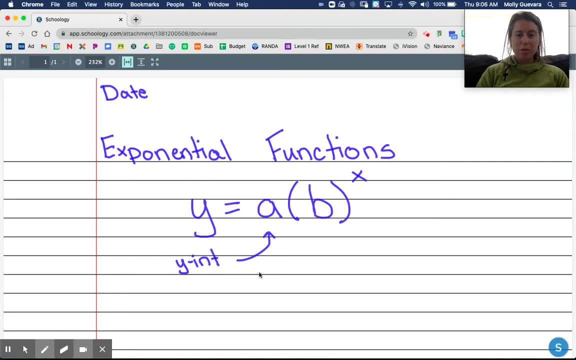 Represents the y-intercept. and remember, if there's no number written, It's just a 1. Okay, B is the base of my exponent and that is my multiplier. That means that is what I'm multiplying by every single time. So really, what we're looking at here in 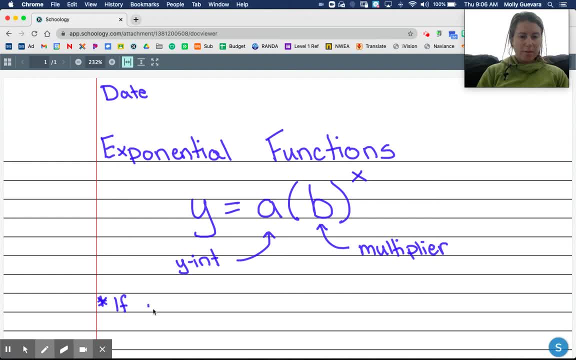 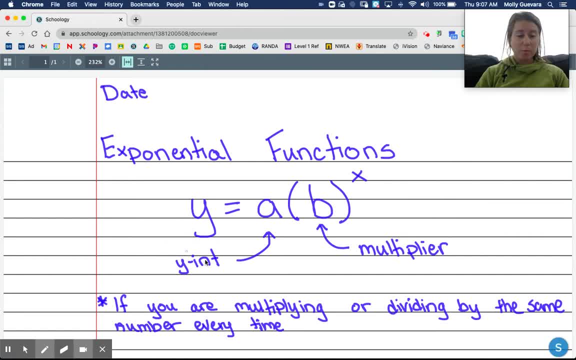 By 4, divided by 4, divided by 4. so every single time you're multiplying by the same number or dividing by the same number, every time, Then it it is an exponential function. So you need to make sure that That X is up here and I'll finish that. 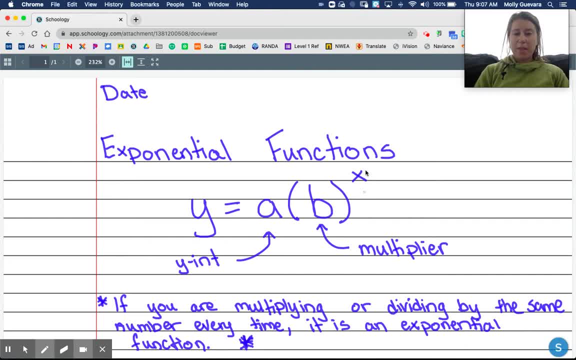 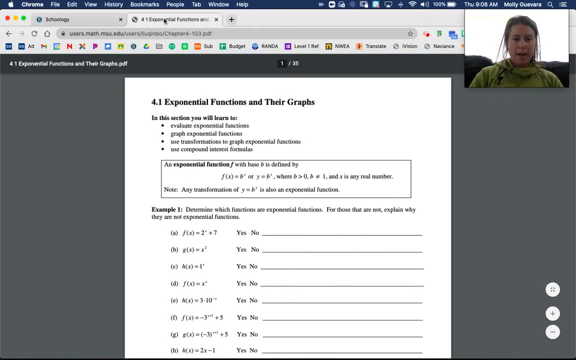 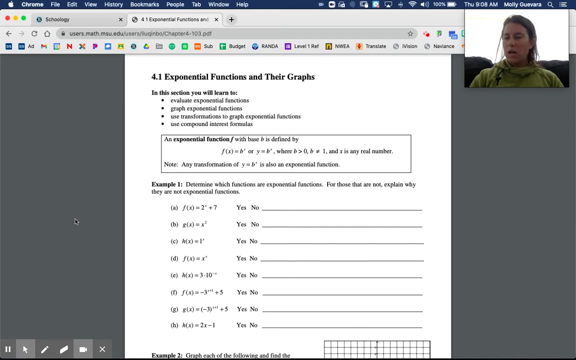 that That X is up here in the exponent Okay. so we're going to look at a couple examples here of You know whether or not something is an exponential function at. Okay, so let's look here. you should have this access to these notes, either in your packet or some other way. 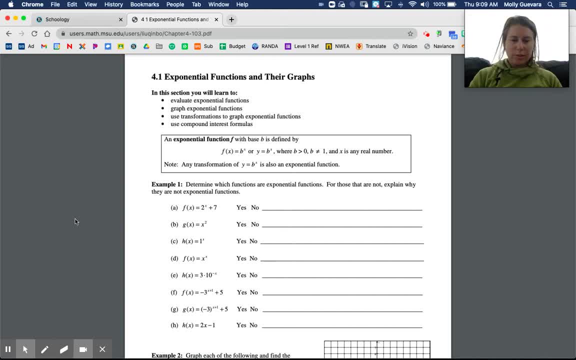 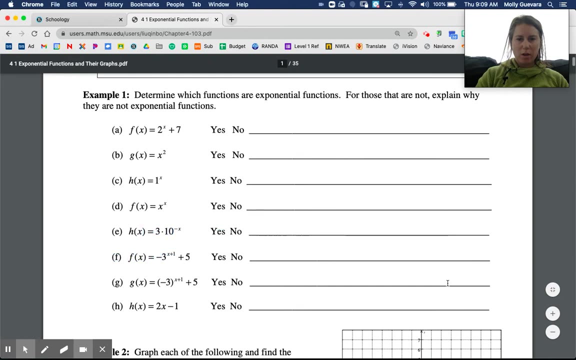 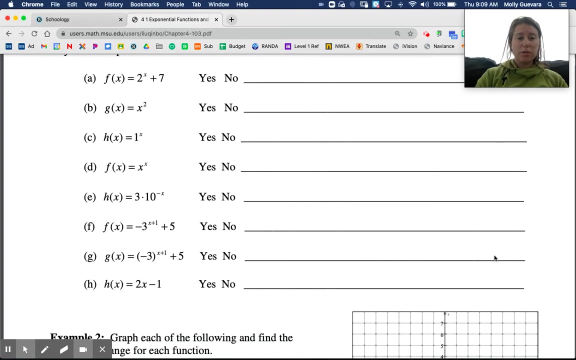 so what we're gonna do here is we are going to go down and we're going to scroll down. okay, we're gonna determine whether or not these are these in example one are functions or not, or exponential functions, excuse me, okay. and so what we're gonna do is we're just gonna kind of go through and I 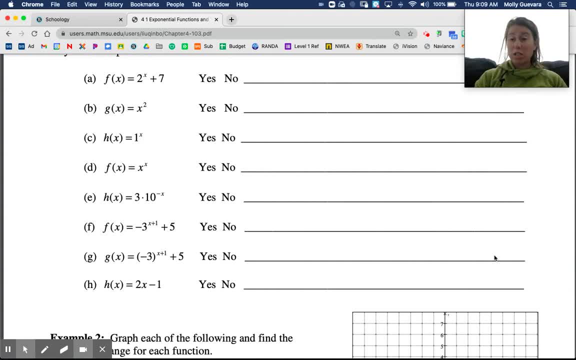 want you guys to try this. so you're gonna hit pause on the video and try it, um, and I want you to see if you can determine whether or not this is an exponential function or not. so just kind of circle: yes, no, and then we can talk about the ones that are not okay. so here I've gone through. 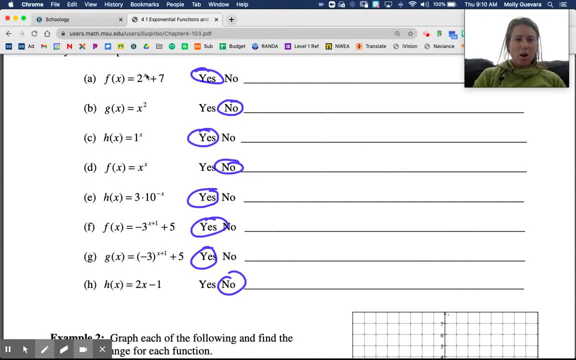 check your answers here. notice that any time though I have an X in the exponent, it is not, or it is an exponential function. X cannot be in the base. so, like here on B, see how it's x squared- the X is a base, not a exponent. so this is not, and this is actually a quadratic. okay, so that's. 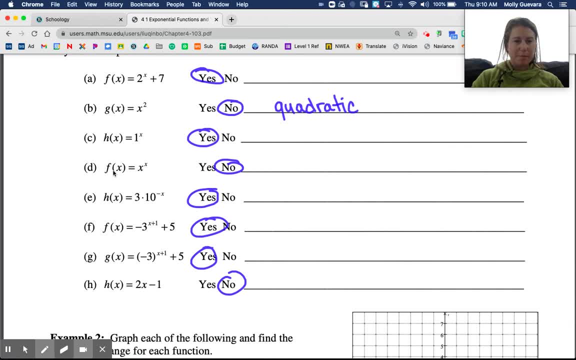 a quadratic function instead. right, because x squared makes a parabola for D. it's no, because even though the X is in the exponent, it's not a quadratic function. so that's a quadratic function. it's also down here in the base. okay, so you cannot also have X in the base? oops, have. that is the. 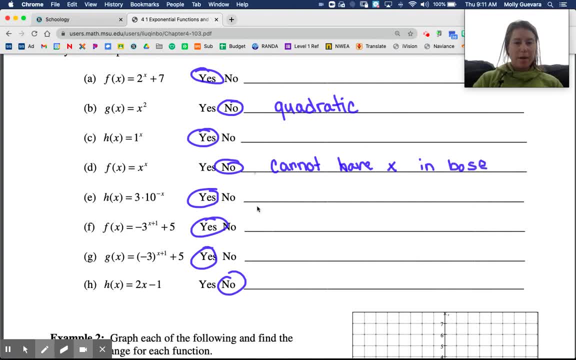 reason why D is not and then H. okay, here, X is not an exponent, it's down here with the two, and this is a linear function. that is a straight line. so again, anytime that you have that X in the exponent, you're looking at an exponential function. so what we're gonna do is we're gonna 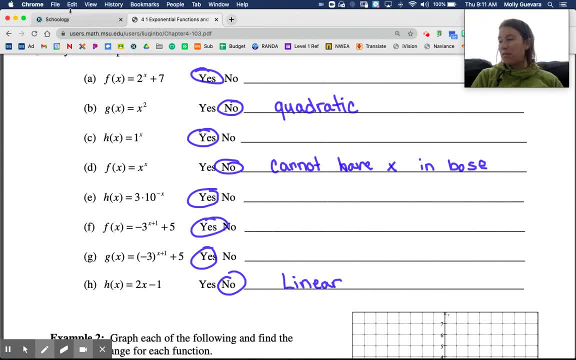 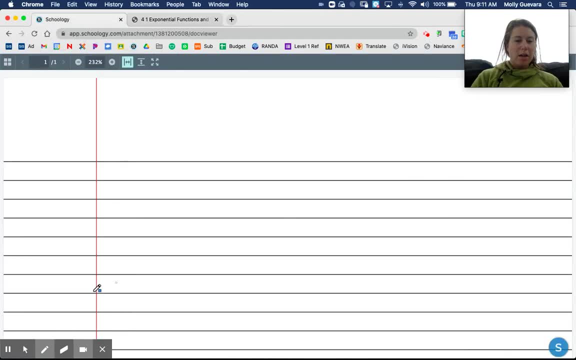 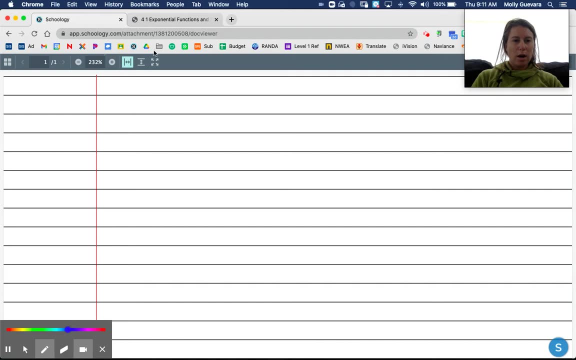 look at the graphs of a exponential function and what makes it hard? I'm we're gonna go back into our notebook here. what makes the graphs hard is that it depends on the base. okay, so the graph of Y is equal to a times B to the X changes depending on B. so that's what makes it a little. 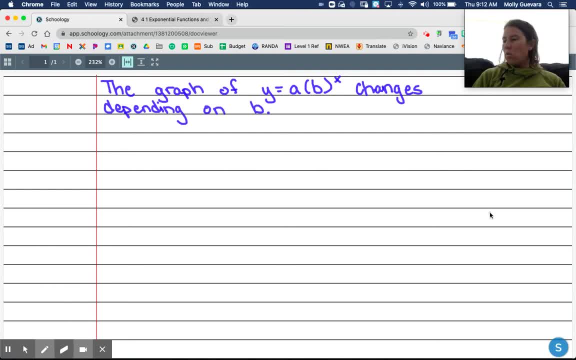 bit more difficult. but what we're gonna do is we're gonna go through an example and then I'm going to give you kind of like the parent quote-unquote parent graph points that you can always use to help you graph the exponential function. so again, in your packet you should have, hopefully, some blank graphs. you only need one of these, so do. 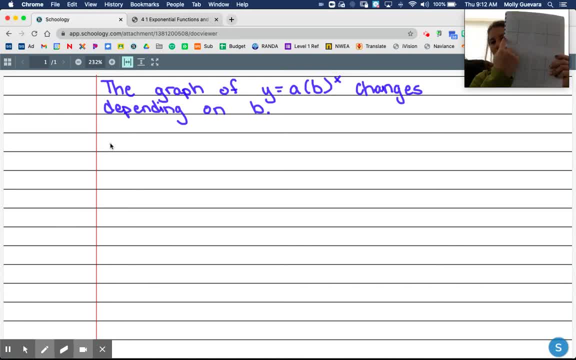 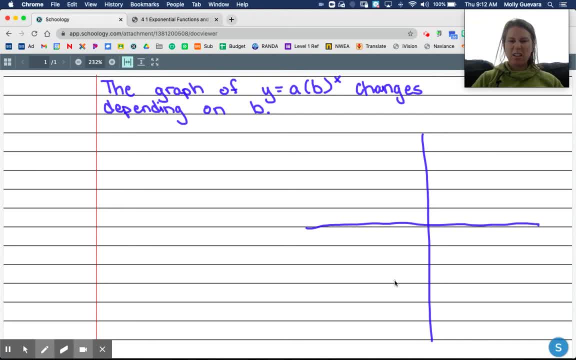 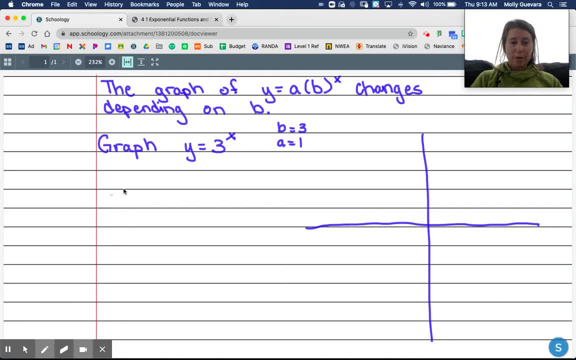 number written out out here so that a is just 1, so we can make an XY table. wasn't very straight, but that's okay and kind of go down to the list. right, if I plug in 0 for X, I'm gonna do it over here. that gets me 3 to the 0. well, anything to. 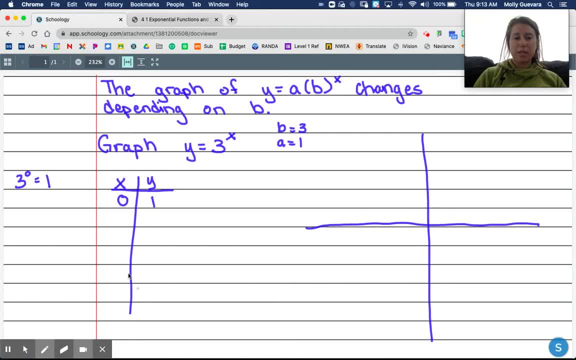 the 0 is just 1. so that gives me a point of 0 comma 1. if I plug in 1 gets me 3 to the 1, and well, 3 to the 1 is just 3. I plug in 2 gets me 3 squared, which is 9. I can keep going. if I plug in. 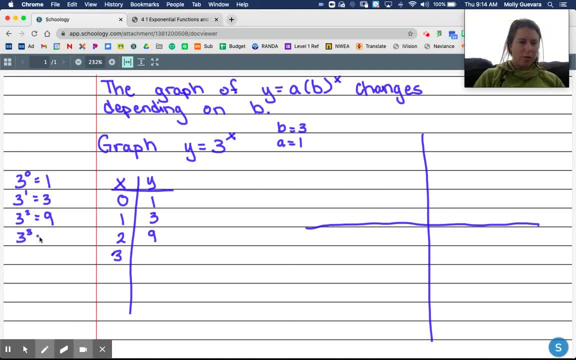 3. it'll get me 3 to the 3rd, which is 27, which is very unlikely. it will fit on the graph right? what about if I plug in negative 1, 3 to the negative 1, and then I plug in 3 to the negative 1, and then 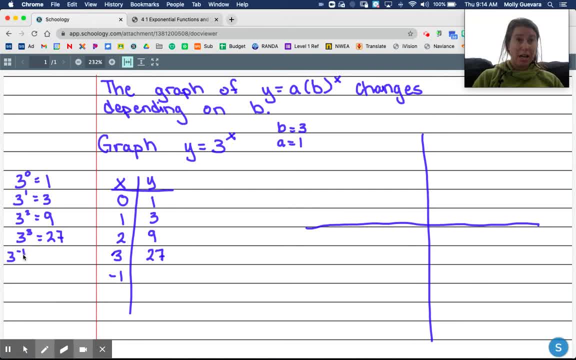 the second thing that might follow up is: what about if I plug in negative 1, 3 to the consider value? so that is just gegangen. so well, 3 to the negative 1, 1 really gives me negative 3, so we have to remember our exponent rules. I cannot have a negative 1 exponent, so this: 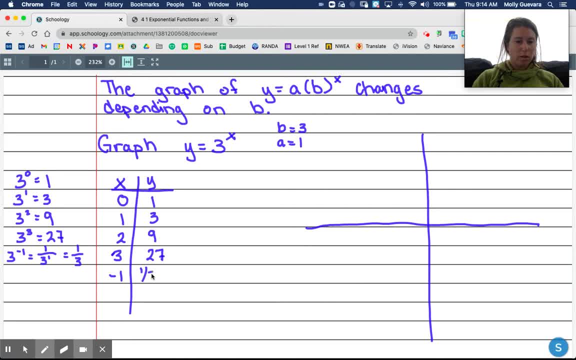 becomes 1 over 3 to the positive 1. well, 3 to the positive 1 is just 3, so you get 1 over 30, so you get one-third. okay, what about negative 2? 3 to the negative, 2 again I. 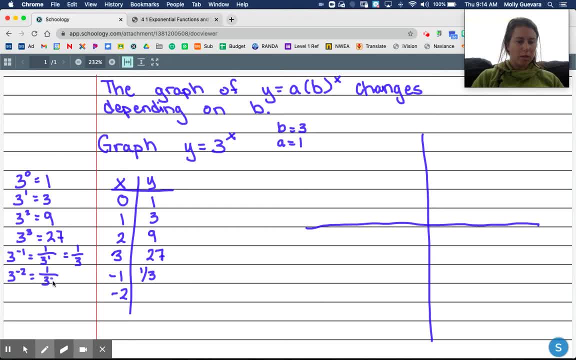 can't have a negative exponent, so it becomes 1 cut over 2, because I need to är to theborough, 就是 1 over 3 squared right. The 2 becomes a positive when I move it to the bottom And 3 squared is 9, so I get 1 ninth. 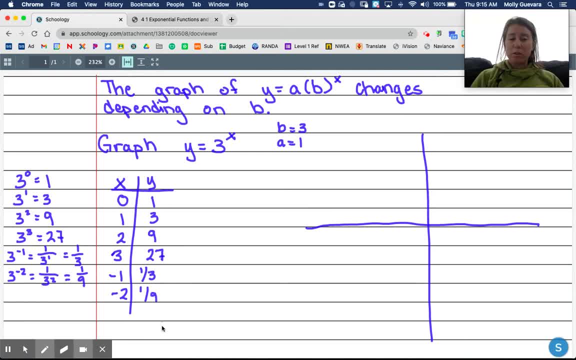 And I could keep going, but negative 3 would be 1 over 27, and that doesn't sound like something I'm very excited to graph. So this kind of gives me my points to then graph it. I'm going to go ahead and graph it. 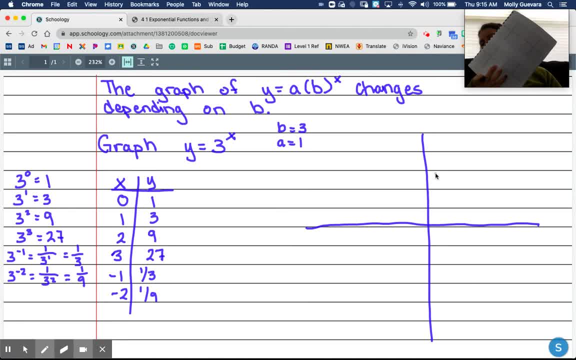 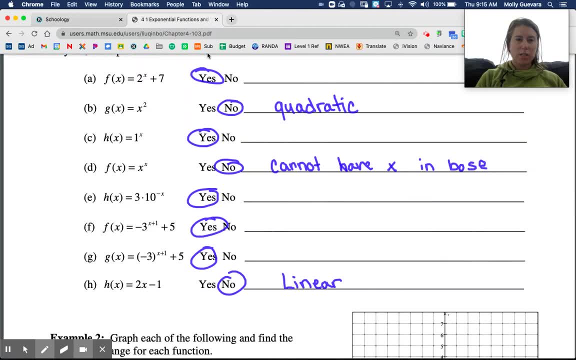 So go ahead and plop that on your graph that you glued in. okay, I don't have one of those graphs, so I'm just going to show you how to do it on here. So don't actually do it on this sheet. 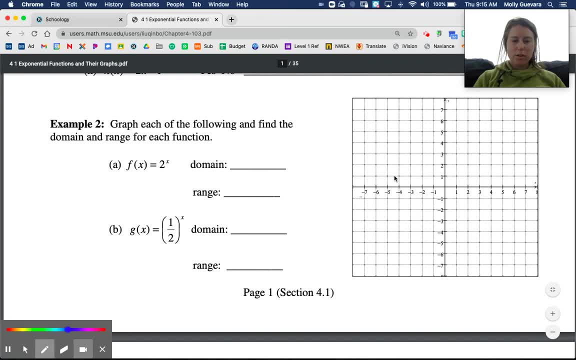 Graph it on that graph that you glued in. But just to show you, I have 0, 1,, 1, 3.. 2, 9,- which is up there somewhere- Negative 1, 1. third negative 2.. 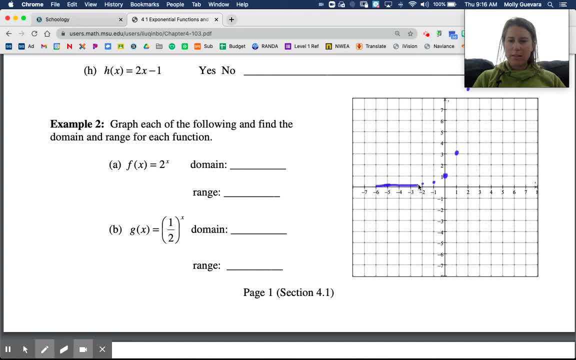 And what actually happens is that there's an asymptote here. Okay, Think about it. If I'm going to the left, I'm dividing by 3, right, If I'm going this way, I'm dividing by 3, dividing by 3, dividing by 3.. 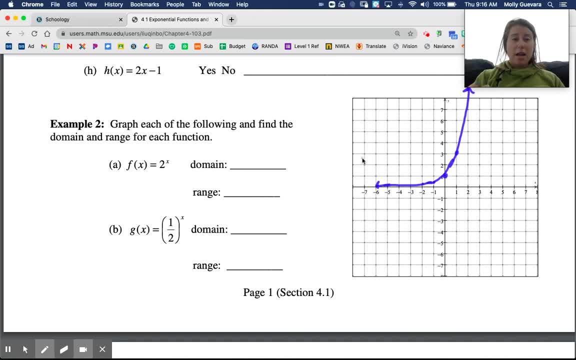 If I keep dividing by 3, will I ever get to 0?? And if we, If we really think about it, the answer is no. The only way I can get to 0 is if I do 0 divided by something right. 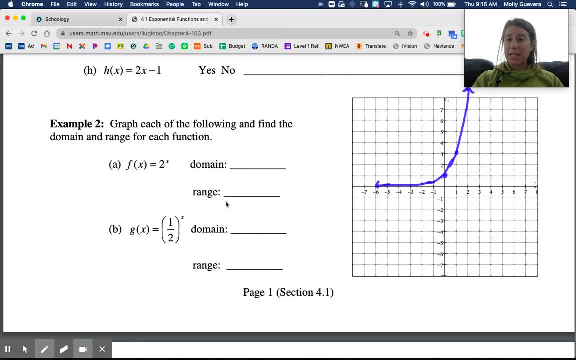 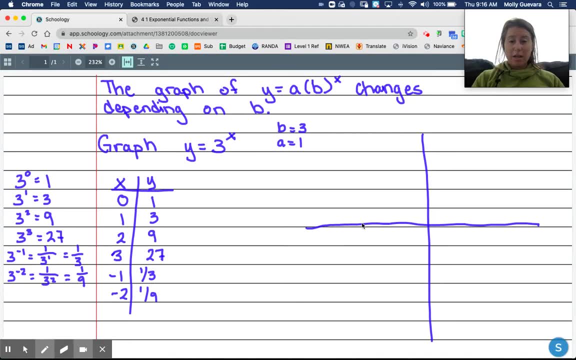 And so, because I never get to 0,, it'll just keep getting smaller, smaller, smaller And I get infinitely close to 0, but I can never get to 0.. Okay, So my graph is doing something like this, more or less. 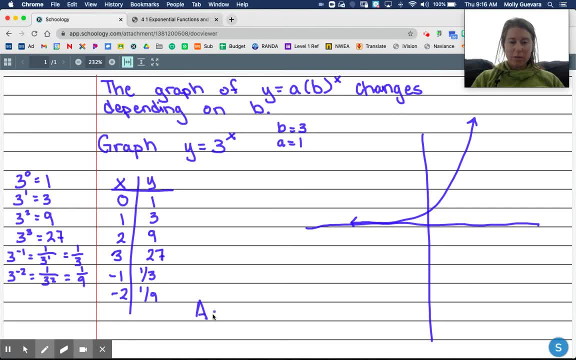 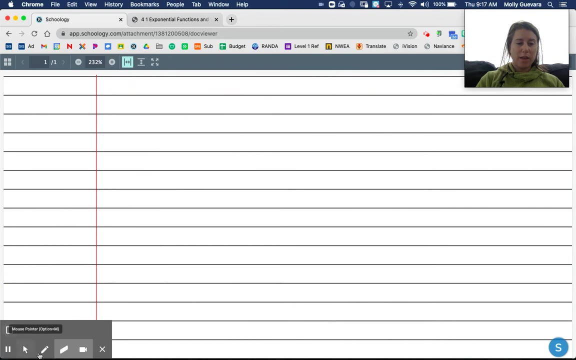 And so the thing to notice is that there's an asymptote On the x-axis. Okay, so there's an asymptote on the x-axis. So what I want to show you now is kind of like the general. how do we graph? y is equal to b to the x, right? 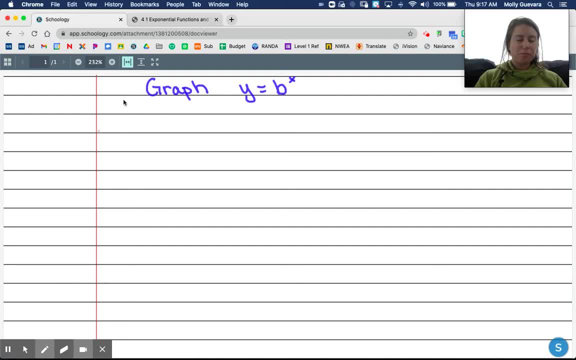 We're going to go ahead And just say that a is 1 here. Okay, so I want to show you the points. First of all, there's an asymptote- Right, We just wrote that on the x-axis. As long as that graph has not been moved up or down, there's an asymptote on the x-axis. 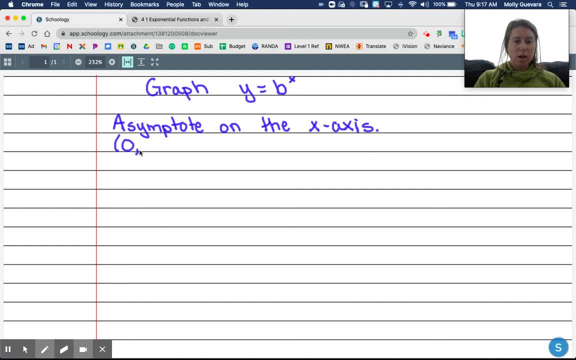 And I'm going to have points at 0, 1.. That will always be a point in this graph, No matter what b is. Then I'm going to have a point at 1, b. So if b is 3, it would be 1, 3.. 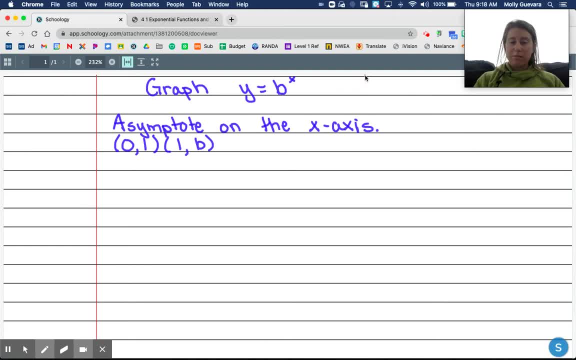 If b is 4,, it would be 1, 4.. Right, Then I'm going to have a point at 2, b squared. So you know, if b is 3, it'll be 2, 9.. 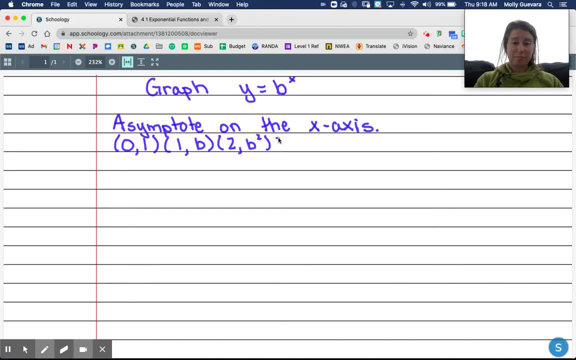 If b is 4, it'll be 2, 16.. You can continue this and say 3, b cubed. Most of the time that will not fit on the graph. And then we can go the other way. We can say negative 1,, 1 over b. 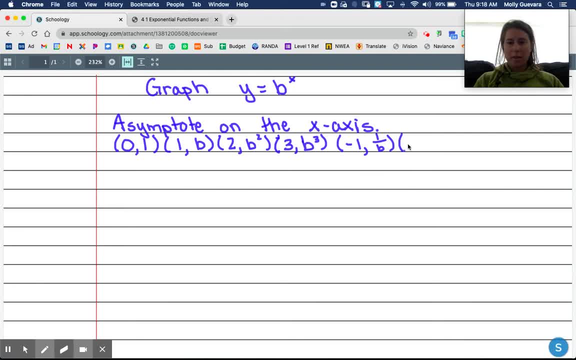 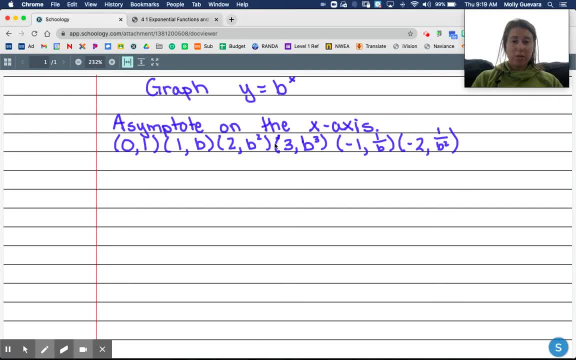 But this kind of is the general idea of how to graph an exponential function. So what I want you to do now is we're going to go back to our little noteshift in our packet. I know we're going back and forth a lot. 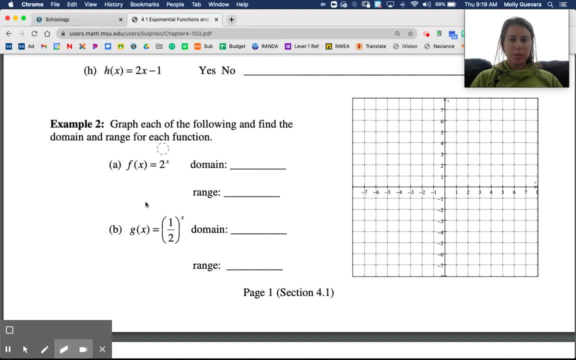 And I want you guys to do example two. So it says: graph each of the following and find the domain and range for each function. So use those points that I just gave you, okay, and see if you can. graph. f of x equals 2 to the x. 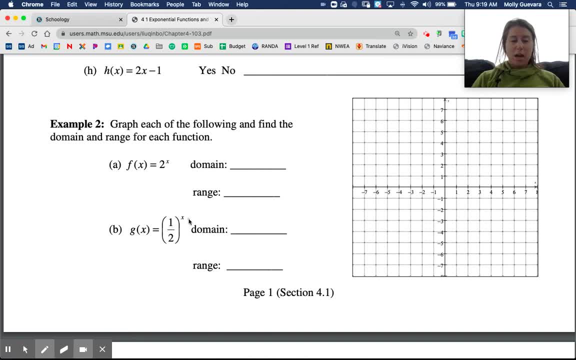 See if you can. graph: g of x equals 1 half to the x. So go ahead, pause the video, use those points I just gave you, give it a try and then, when you're ready to review it, you can hit play and we'll go over it. 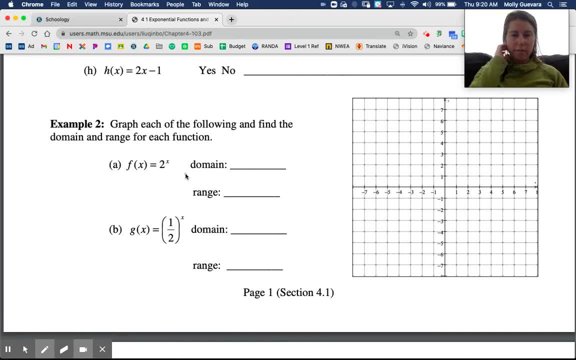 Okay, so let's go over these. Hopefully you gave it a shot, But I'm going to do these in two different colors, since we're going to graph them both on the same graph. okay, So f of x equals 2 to the x. 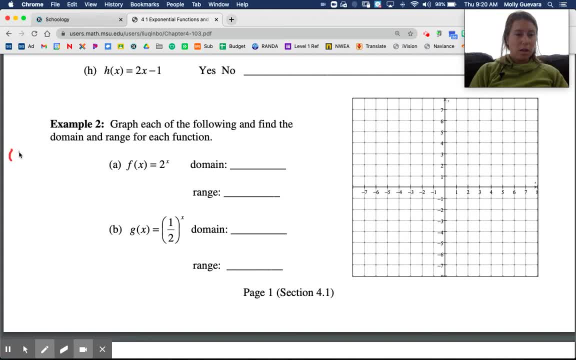 So I know that I'm going to have a point because a is 1, right, So a equals 1.. b here my base is 2.. So I know I'm going to have a point at 0, 1, right here. 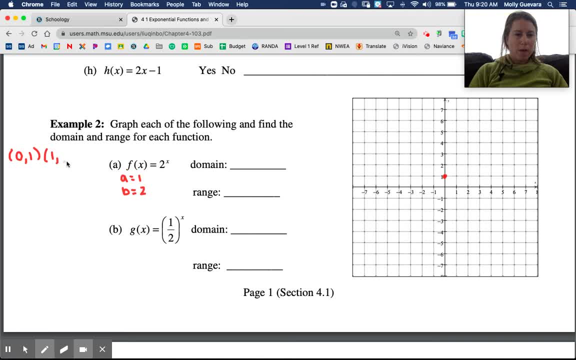 Okay, then I'm going to have a point at 1, b. Well, b b is 2,, so 1, b, so 1, 2.. Then I'm going to have a point at 2, b, squared. 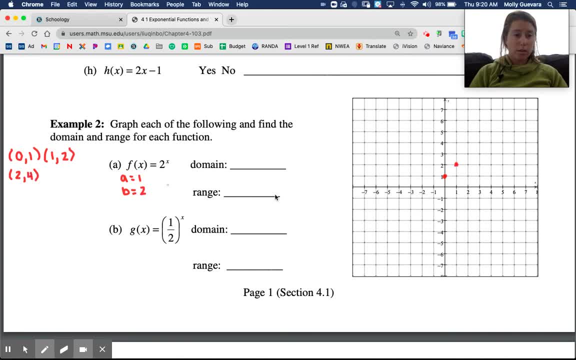 Well, 2 squared is 4, so 2, 4.. Then I'm going to have a point at 3, b cubed, 2 cubed is 8, right, 2 times 2 times 2 is 8.. 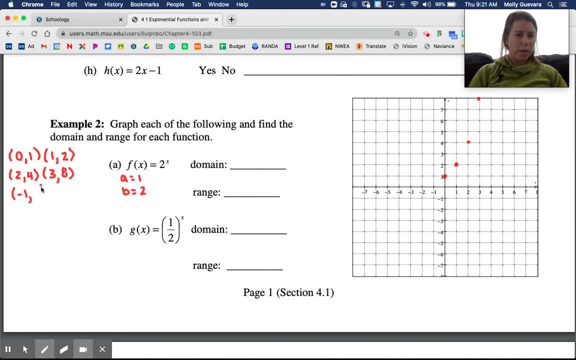 Okay, then I'm going to have a point at negative 1, 1 over b. Well, b is 2.. So negative 1, 1 half is a point. And then I'm also going to have a point at negative 2, 1 over b squared. 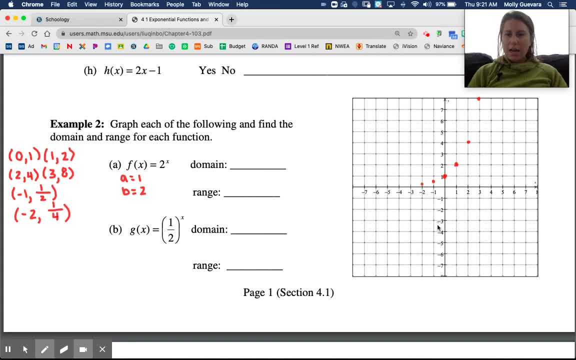 b squared is 4, so 1 fourth, And I can keep going and do 1 eighth, but it just seems like we don't really need it. We can kind of see What this graph looks like now, So I connect it, knowing that there's an asymptote on the x-axis. 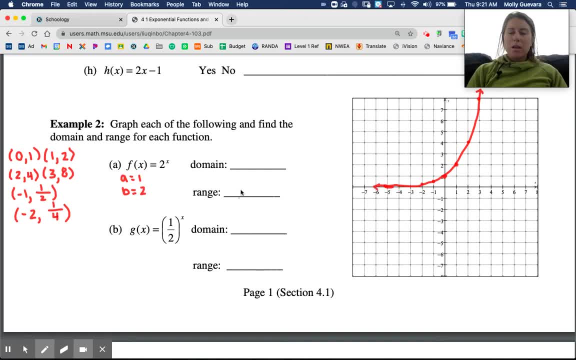 So the graph never crosses the x-axis. Okay, so now let's find the domain and range here. How far to the left does this graph go? Well, there's an arrow, so it keeps going on and on and on. So it goes on to negative infinity. 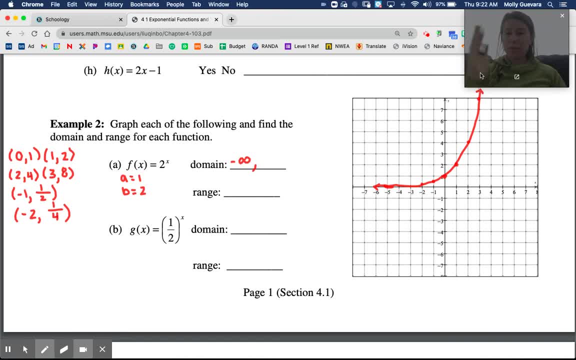 And then, how far to the right does it go? Well, again, it has an arrow, so it keeps going Over, over, over, over, over, over right, So it goes up to positive infinity, And we always use parentheses at infinity. 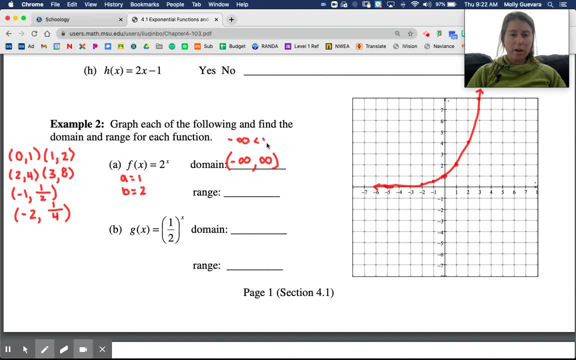 So you can write it like that, Or you can write it like this, Or you can say: x is in the set of all real numbers. All three of those options work. Just pick one. You don't have to write down all three. 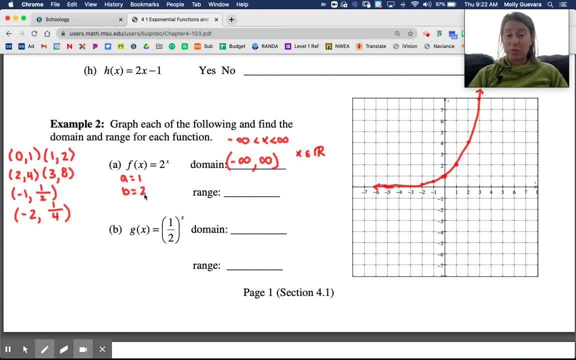 Just pick the one that you like, Or pick the one that you've been using. Okay, my range. What's the lowest that this graph goes? Well, it never, ever ever crosses zero. So the lowest I can get is zero. 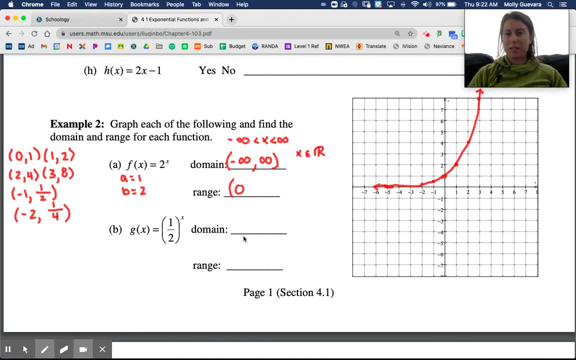 But it doesn't actually ever get to zero, So it's a parenthesis at zero. And then what's the highest that this graph goes? Well, this graph keeps going up and up and up all the way to infinity. So again, you can write it like that: 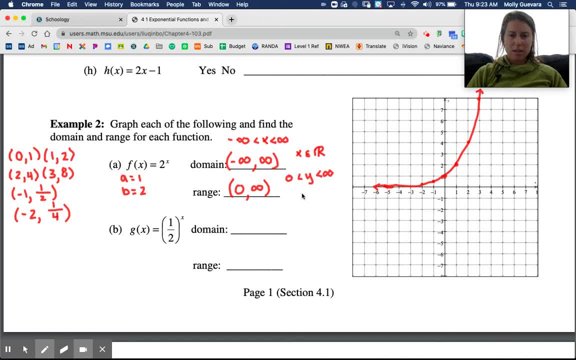 Or you can write it like this Either way. Okay, now let's go ahead And look at g of x. If you haven't tried it yet, this would be a good time to pause it and try it. And we're going to do g of x in a different color. 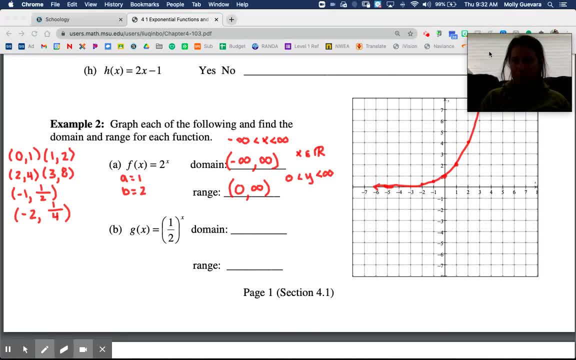 Okay. so now? Uh-oh, How did that happen? I'm all dark, Okay, so now what we're going to do is we're going to look at one half to the x. So again, it's going to be the same thing. 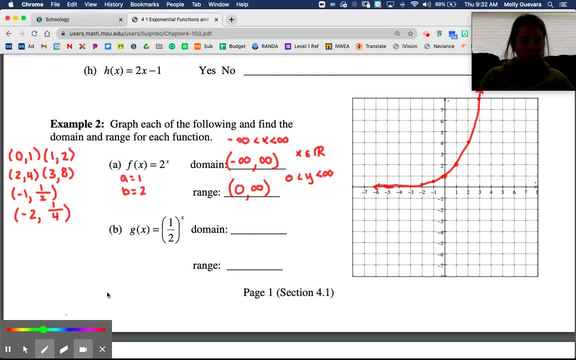 My a is one. right, What's going on? My a, there we go, is one And my b is one half Okay, so I'm going to go through And since a is one, I can say that zero one is going to be a point. 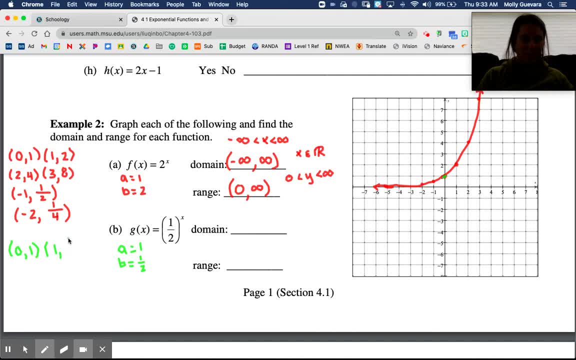 I can also say that one comma b is a point, So it'll be one comma one half There. Two comma b squared. Okay, so one half Two comma b squared is the same thing as one squared over two squared, which is one over four. 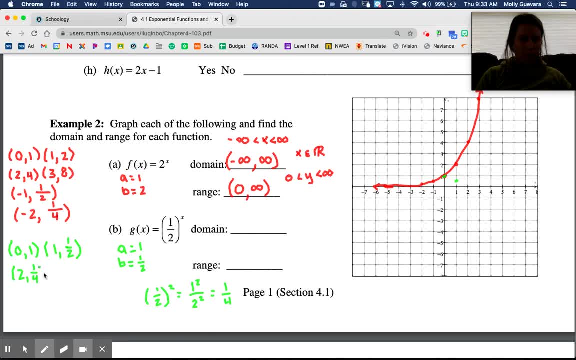 Okay, so two comma. one fourth is a point, And then I can keep going and get one eighth, but I'm not going to, So let's go the opposite way now. Negative one comma. My pen is all jumpy, My screen's all dark. 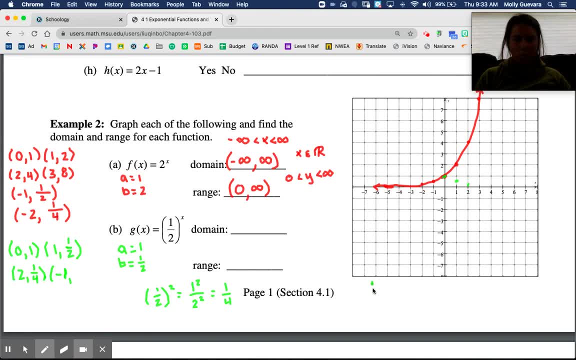 Okay so. So it's one over one half, Right at negative one. So watch what happens when I write it the other way: One divided by one half, So I make the one a fraction. Now I have dividing fractions, So it's copy dot flip. 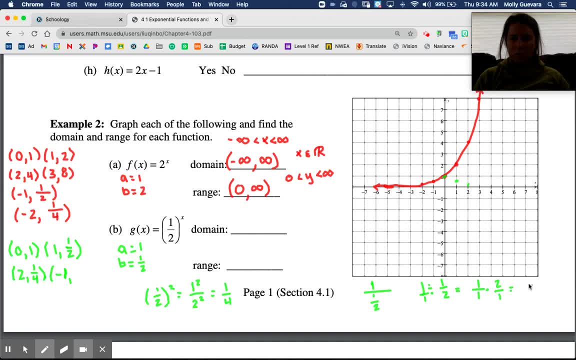 Okay, So I get two. So negative one comma two is a point At negative two. it's one over b squared, So now let's get rid of this. I know that b squared is one fourth, So it'll be one over one fourth. 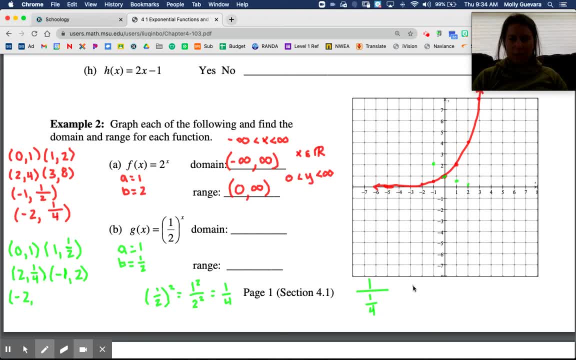 And I do the same thing. So I get one over one half One divided by a one fourth, And I copy, dot, flip And I get four. So it's negative two comma four, And I could keep going. Okay, Negative three would be. 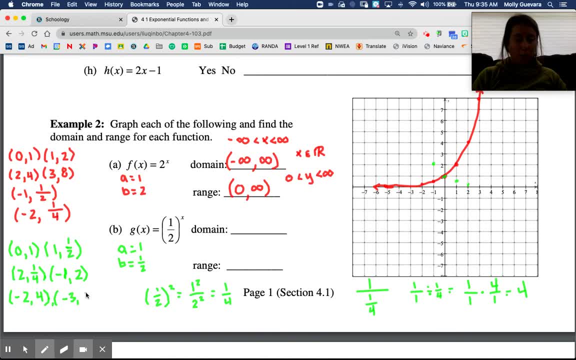 One over B to the third, which gives me eight. So it's really just the same points up here, Just flipped over the y-axis. Oh, I didn't get this. one, Two, four And then negative three, eight. 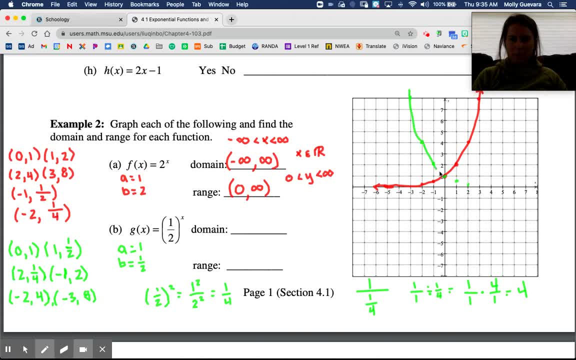 So it's the same graph as the red one. It's just: oh boy, sorry, It's just flipped over the x-axis And that's where it's going. So it's just like this. It's just like this, And I'm looking at the graph. 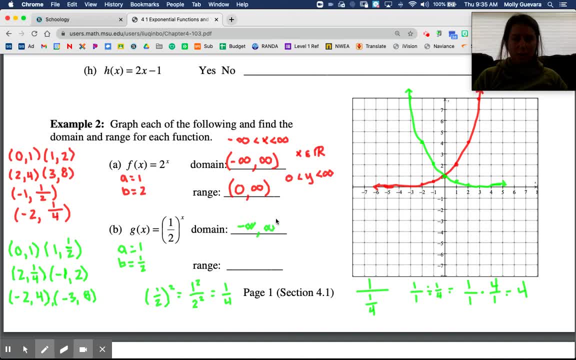 And because it's the same graph, it's not just one over b squared And it's gonna be a really long graph, But it's just a María that's broken, But it's just one over one, So I'm gonna put this here. 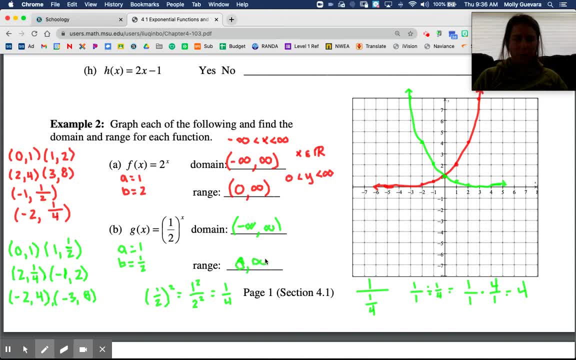 So here it's a, two, two, three. This is the half, This is the half. It's going to be two over b squared. This is a. one over b squared are the same regardless. Domain will always be negative. infinity to infinity. and then your range. 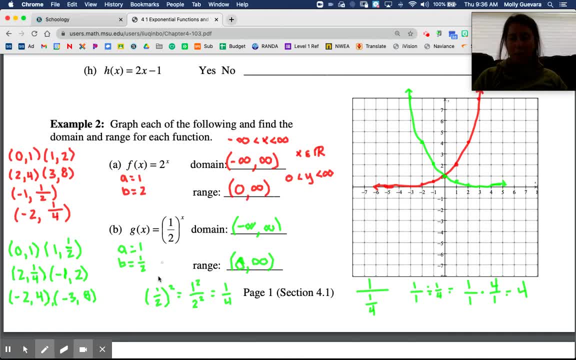 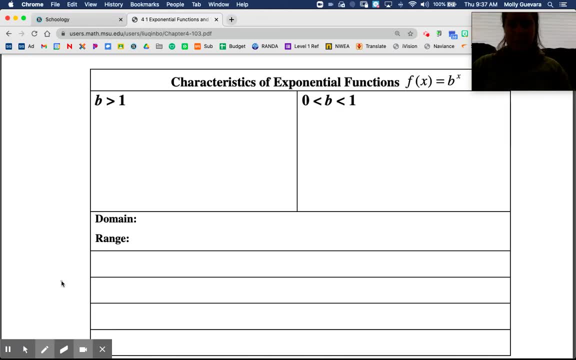 will only change if you shift the graph up and down. Okay, so the last thing that we're going to talk about here is: what happened? what did we notice that happened when b was greater than 1, like when we graphed the 2 to the x, and what happened? what did we notice that happened when? 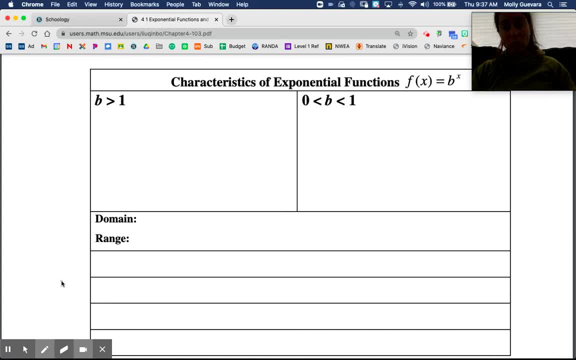 b was less than 1, or between 1 and 0,, like when we graphed for 1 half to the x. So when b was greater than 1, that was like my. the one that we did that was like: f of x is equal to 2 to the x. 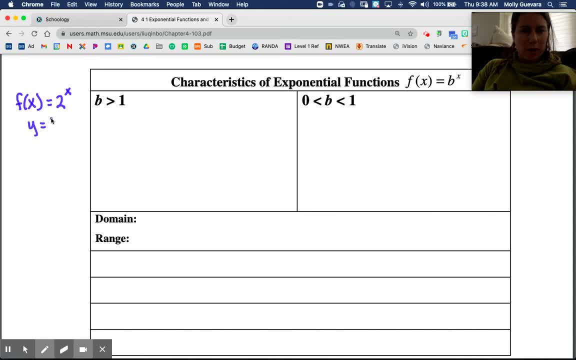 or we also graphed ourselves: y equals 3 to the x right, Anything where b is greater than 1.. So what's going to happen? there is, the graph increases from left to right. My pen doesn't want to work today, that's okay. Okay, so the graph is going to increase from left. 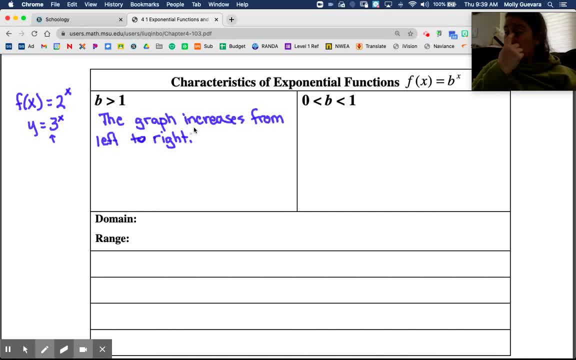 to right. So if we look at that graph of 3 to the x, it's going up. we look at that graph of 2 to the x, it's going up from left to right. okay, So I guess here we can write those examples. 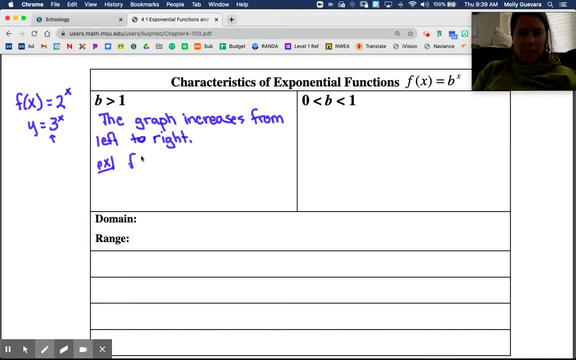 We don't have to write it on the outside like I did. So that f of x is equal to 2 to the x will be increasing from left to right. If I have, y is equal to 5 times 3 to the x. 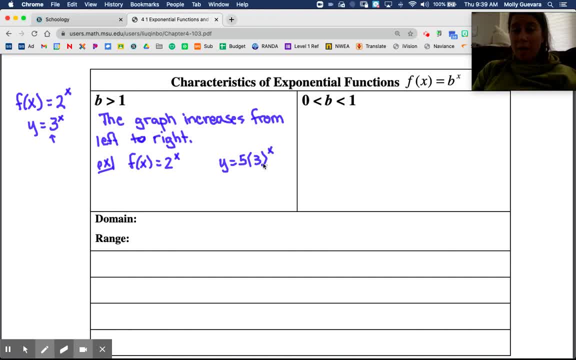 this is going to be increasing from left to right. a is 5 and then b is 3, so b is greater than 1.. And if I have something like negative 1, half 4 to the x, it's going to be increasing from left to right. 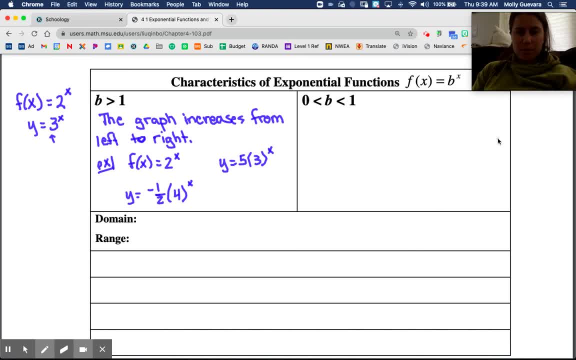 b is greater than 1.. What about if I do 0 is less than b is less than 1?? So this is like whenever you have a fraction that's less than 1, okay, So that's going to be increasing from left to right. 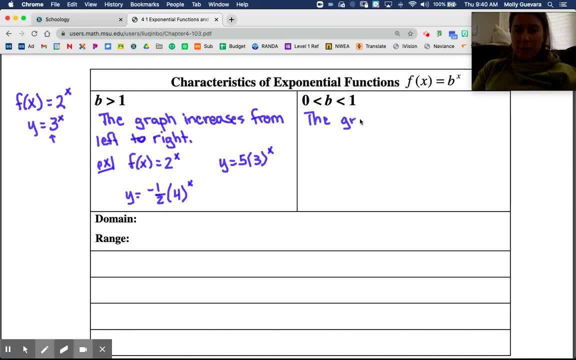 So here you're going to get that. the graph decreases from left to right. It looks like I'm writing with like a chisel or something From left to right. Okay, so this was that 1 half x that we did, right. 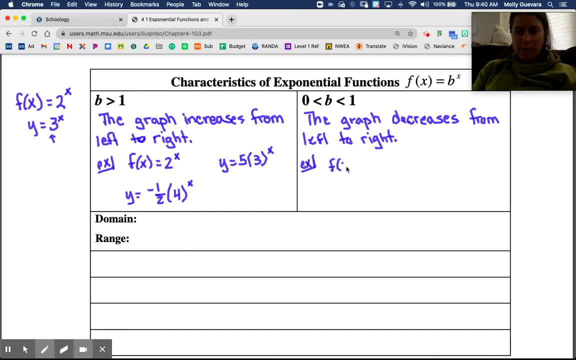 That was on the previous page, So that f of x equals 1 half x or 1 third or 1 fourth or whatever right y. you could say y is equal to 3 times 1 fourth. To the x you can say f of x equal to negative 2 times 1 third x right. 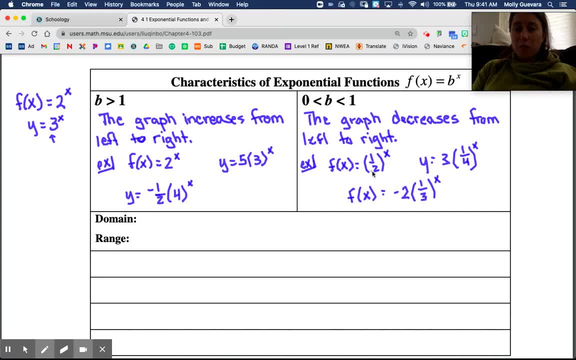 So this is when you're going to have fractions that are less than 1 in as your base, right? So inside the parentheses, or as your base? Okay, the domain of exponential functions: we just talked about it. The domain is always going to be negative: infinity to infinity. okay. 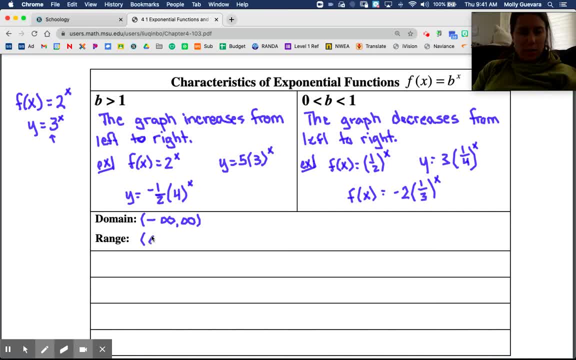 And then the range is always going to be 0,. oh boy, 0 to infinity. But we're going to make a little note here. I'm going to say: unless graph is moved, Holy moly, You guys can't even read my handwriting. 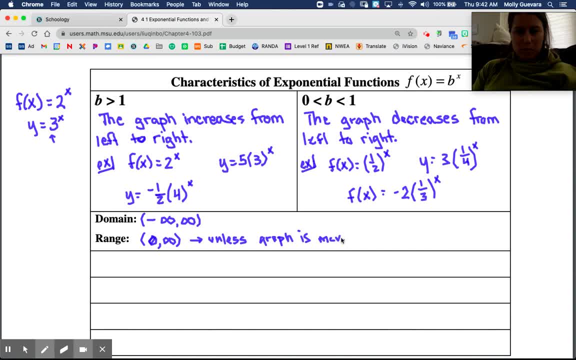 Is moved, Not left or right- Sorry, I'm getting distracted by my bad handwriting- So unless the graph is moved up or down, It's funny, it like won't make like. let me make a curve. Everything is like a straight line. 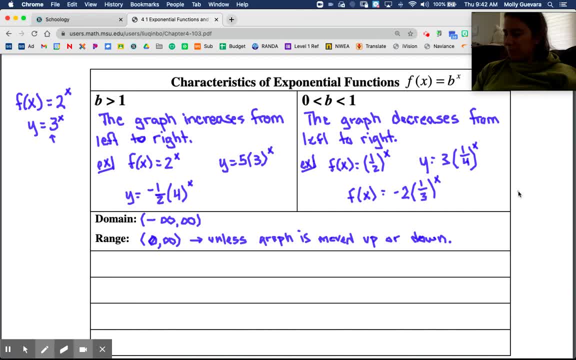 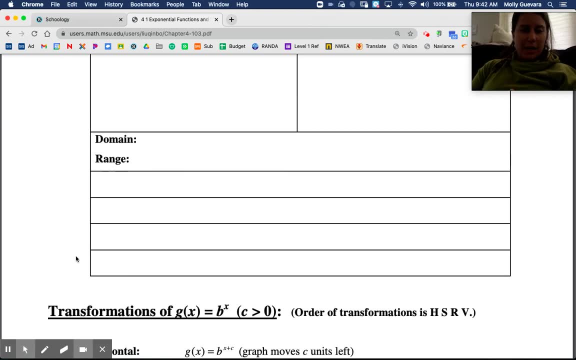 Okay, so unless the graph is moved up or down, that will change the range, But for the most part it's going to be 0 to infinity, And then you adjust it if it's been moved up or down. And then the last thing that we're going to look at here, in these four little boxes, 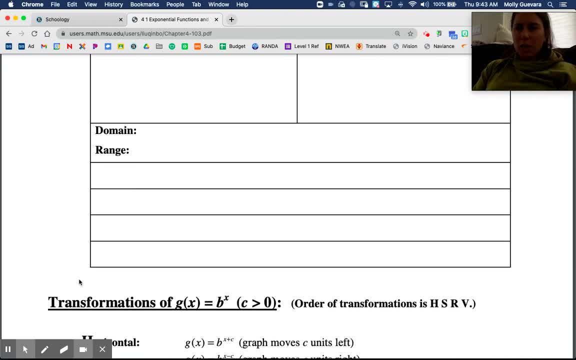 are some things that are going to be really helpful For us, some tips and tricks, right? So I want to just point out that multiplying by 1 over x, right, So if I have like one third or one half or whatever, right. 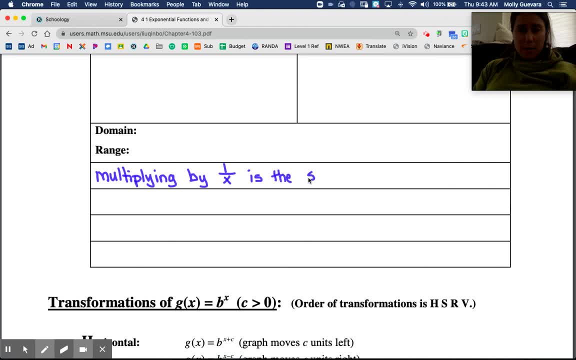 Is the same as dividing by x. So let me show you what I mean by that. So if I have the equation, let's say y is equal to 3 times 1 half x. That tells me that I multiply by 1 half every time, right? 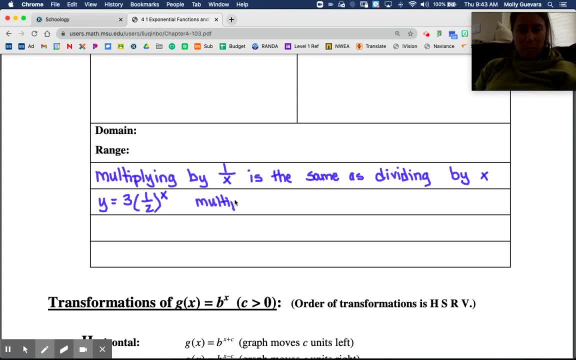 So multiplying by 0.5, multiplying by 0.5, or multiplying by 1 half, So multiplying by 1 half. Sometimes it's like kind of hard to do. You're like, okay, what's negative 1 times or right. 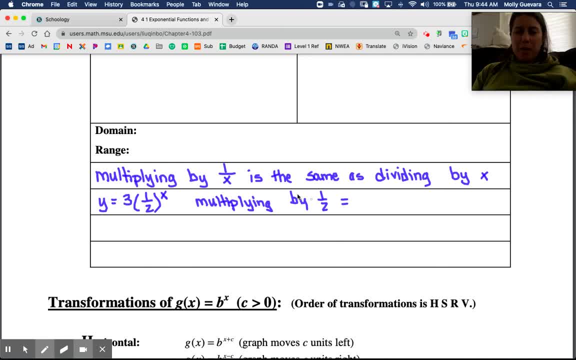 Like 1 over 1 half or whatever. Like multiplying by 1 half sometimes isn't the easiest, So we can also think of this as the same thing as dividing by 2.. So if I'm like, okay, multiplying by 1 half every time, 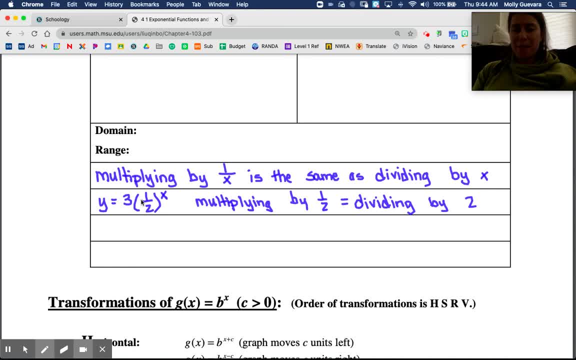 I can also think of it. okay, I'm dividing by 2 every time And that makes it a little bit easier, Easier to think about. okay, Same thing. what if I have, like f of x equals 2 times 1 third of x, right? 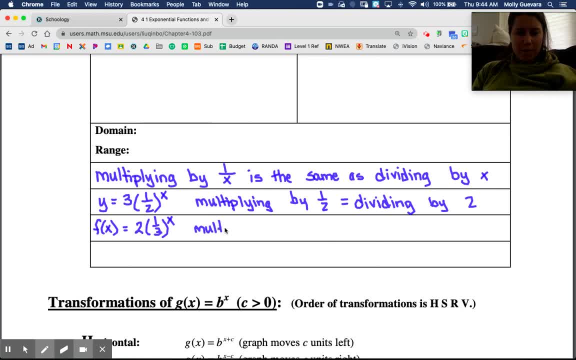 So here I'm like: okay, I'm multiplying by 1 third. every time That's kind of hard to think about Multiplying by 1 third, okay. So you're like, okay, Okay, I multiply by 1 third to get my next point. 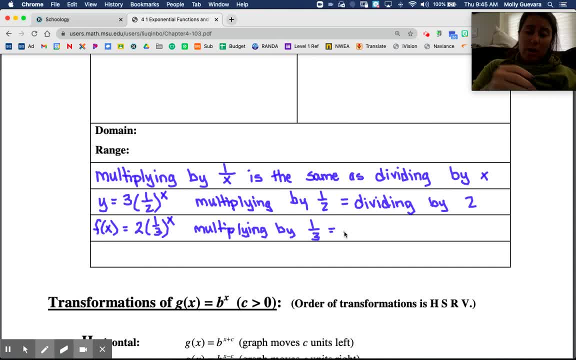 and then multiply by 1 third to get my next point and my next point and my next point. Or you can just think of it as: hey, I'm dividing by 3 every time. Sometimes it's helpful to think about it as multiplying. 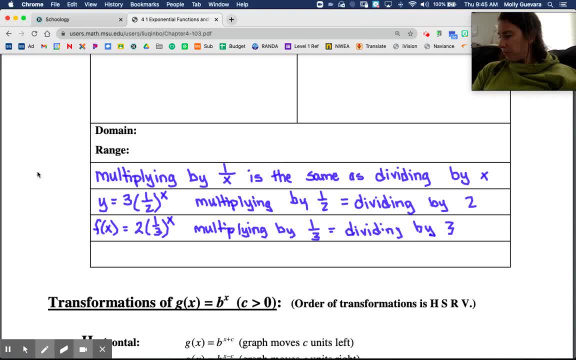 but sometimes it's helpful for us to think about it as dividing And then, like you, also can think about it the other way around. Okay, Okay, The other way. like what if I have, like, y equals 4 times 2 to the x right?